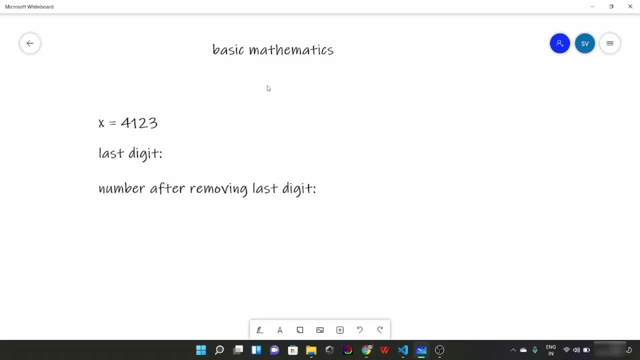 so, before jumping to some topics, I would want you guys to be familiarized with two mathematic you know operations. one is divide, which looks something like this straight line, you know, right, right. and when a percent sign like all right. so let me tell you about these through the examples. all right, okay, suppose we have a. 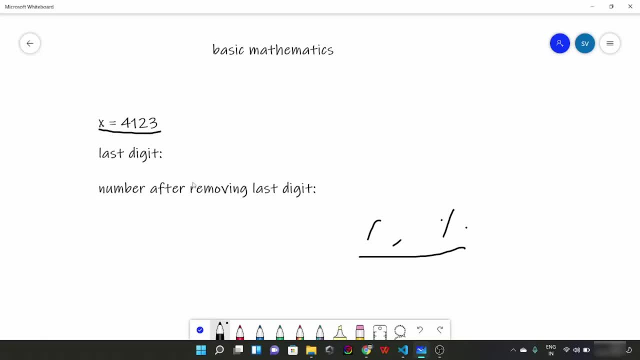 number here, X, which is 4, 1, 2, 3, right, and on the last digit of x, it is what going to be 3, right, and if I ask like, what would be the, what would be the value of X, I remove this 3 formula. so we want 412 right now. can programming or when we are writing a 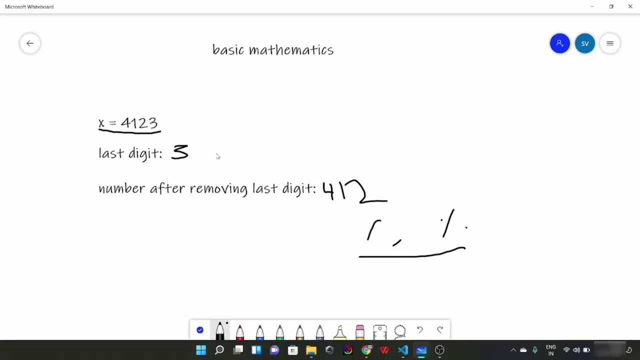 program. how will you find the last digit? so many of you guys, but let me still tell you what we do is we? this is our X, which is variable here, percentage with, then, all right, so what this perfect sign goes. all right, so what, this perfect sign goes. 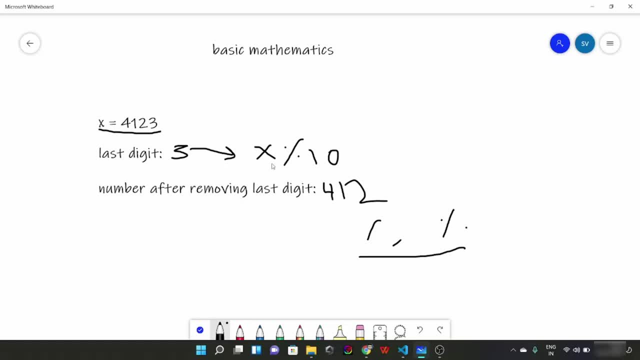 1, 0, 2, 3, all right. why are you submitting a 0, 1, 2, 3, all right, sorry, yes, Z, 11. but can 1, 0, 2, 3, all right. so what's the function of your 0, 1, 2, 3, all right, sorry, yes, Z. and then. 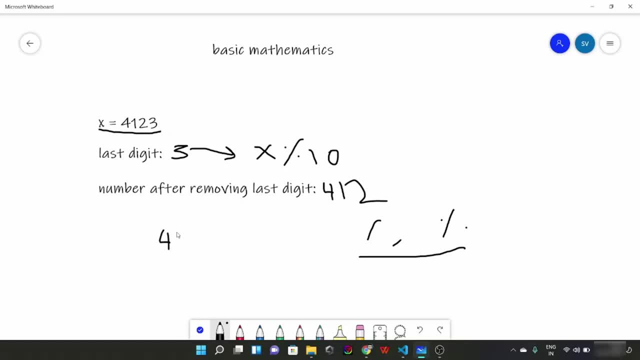 1, 0, 2, 3, all right. so what's the function of your 0, 1, 2, 3, all right. sorry, Z's ess draws an emotional rarity. nature is actually very dependent on the накlars. absolutely onlyvial, or better term than the. 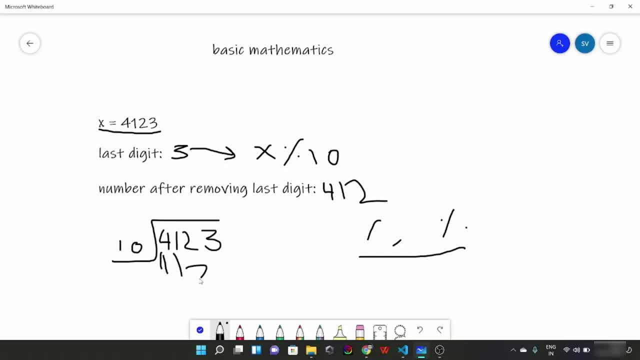 So you know what: 4, 1,, 2, 0, and then that would be 3, and this x percent n would return 3.. Alright, Now another thing I want to ask you guys is how will you like find a number after removing? 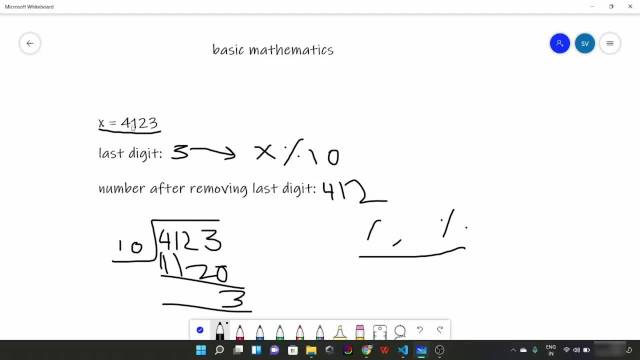 last z. Suppose like x, 4, 1 is 4, 1,, 2, 3 here, and I want answer to be 4, 1, 2.. Then how would you do in programming? So what you will do is you will return x divided by 10, alright. 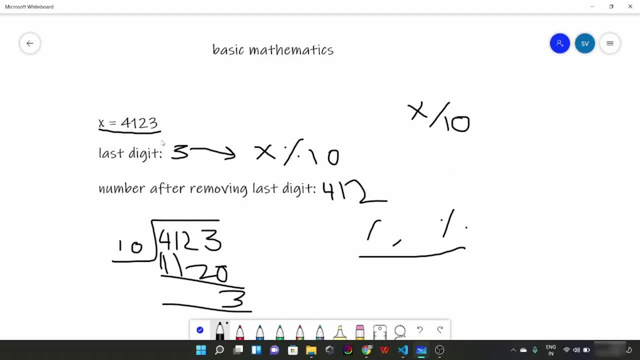 So this is a simple division, which we do alright, Since x is our integer. so x divided by 10, if we store it in our integer variable, x would be what? 412.2.. 412.3.. But since we are storing it, or you know, outputting it in integer form, hence the answer would: 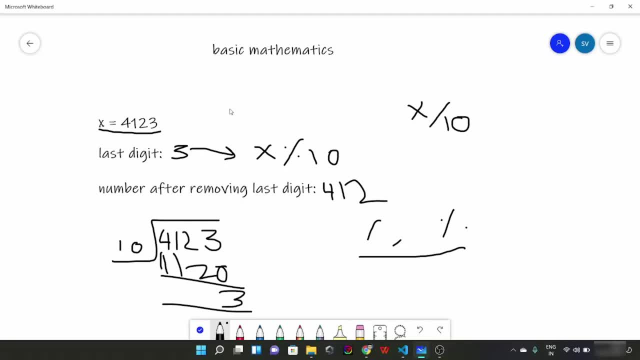 be 412.. Or 412.3.. So the answer would be 412, right, And we will discard the point form, and then the last digit would be discarded and we will get the number 412, alright. So these are the two functions which I wanted to tell you. 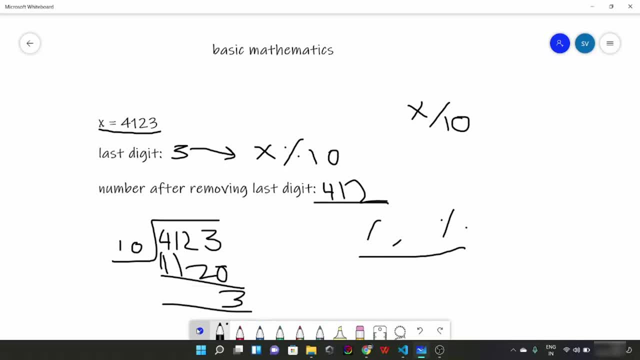 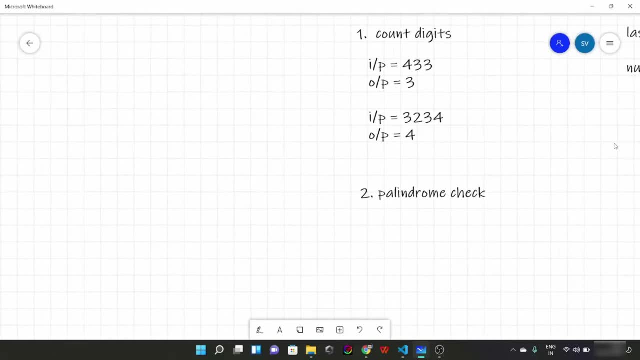 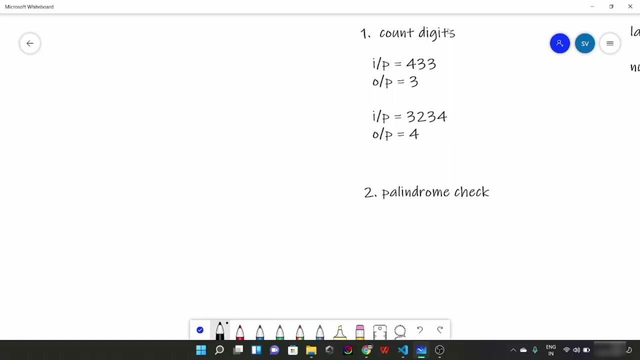 Alright, So it is a very important one. Alright, Now let's jump to some questions. or I would say: yeah, basically there are topics, not questions, with tracking. alright, So this would come handy in future programming questions. okay, Suppose we have to find number of digits in any number. 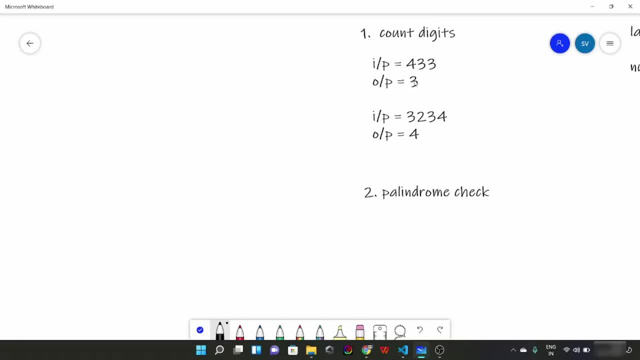 So let's say two digits. Okay, Alright, suppose here our input is 433.. What would be our output? It is going to be 3, right, 1, 2, 3.. Suppose our number is 3,, 2,, 3, 4.. The number of digits here is 4.. 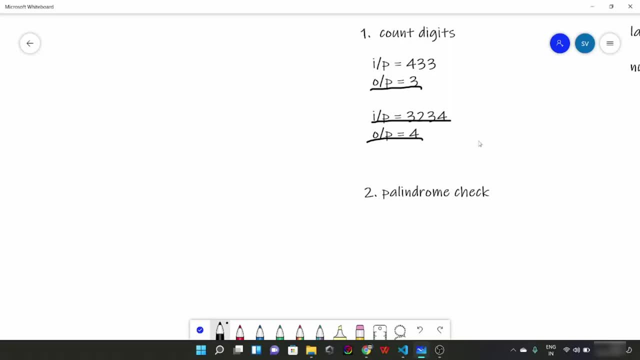 The output would be 1, 4.. Right now, pause this video and try to come up with a solution to find the number of digits. Alright, so here is a very basic and very easy solution. This is going to be a greater solution. 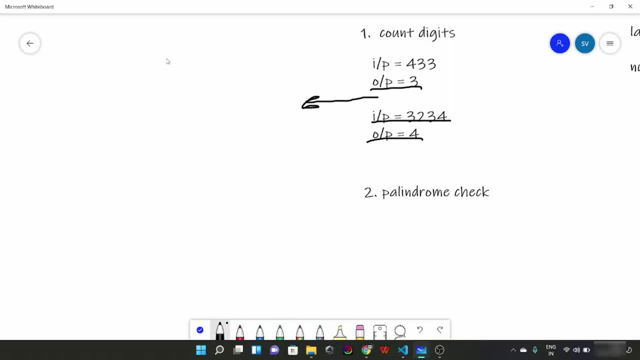 Alright, so what we are going to do is we have number n, which is what? 433, right Now, we will run a loop and we will, you know, going to divide n. We will run n by 10, continuously until n becomes 0.. 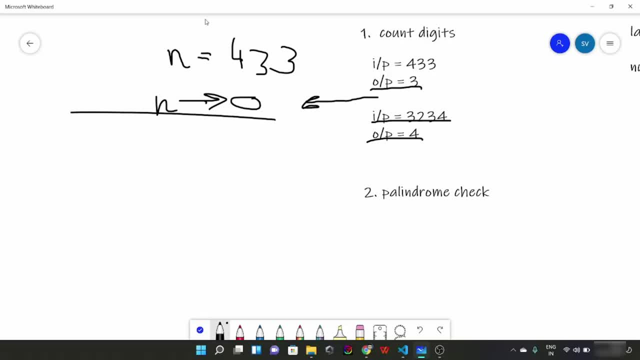 Alright, when this happens, we will come out of the loop and you know we will have a variable count which will show the number of times the loop would run, and that would be an answer, Alright. so let me tell you by doing a dry run. 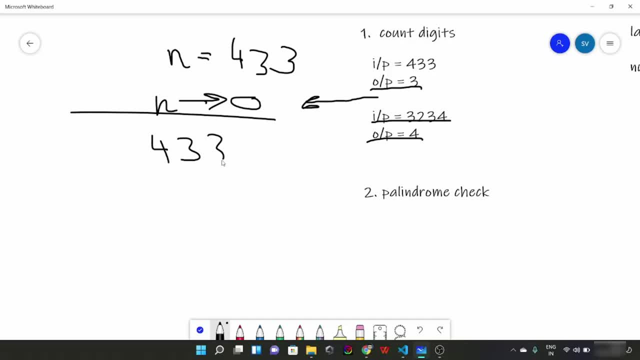 So initially our n is what 433.. 433, suppose our variable, which will have a count, is going to be zero. all right, now, in the first one, what we'll do is we'll divide 433 by 10.. so now our n would be what? 43? 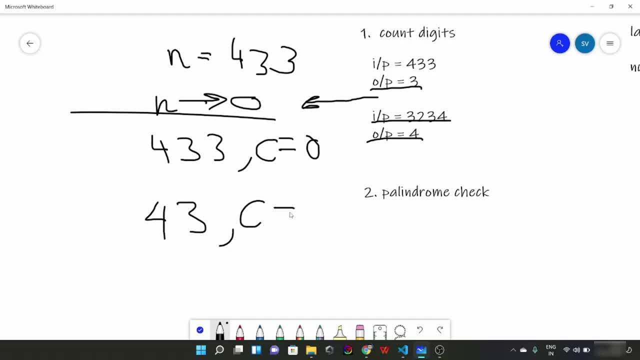 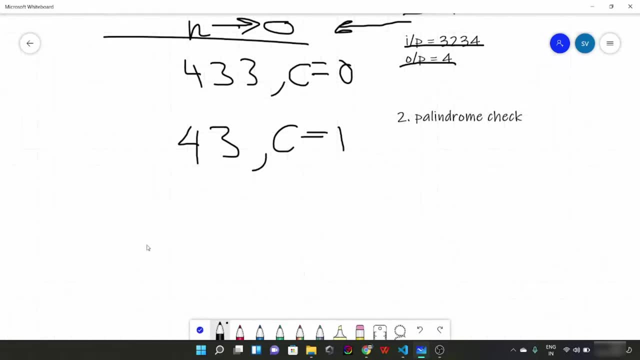 yes, c will become what one? all right. then we'll divide n again by 10. now it will be worth four. c will you know, become two. yes, now what will happen? we'll divide four by ten again. now. now n would be zero and c will become three and as well, and zero will come out of it. all right. 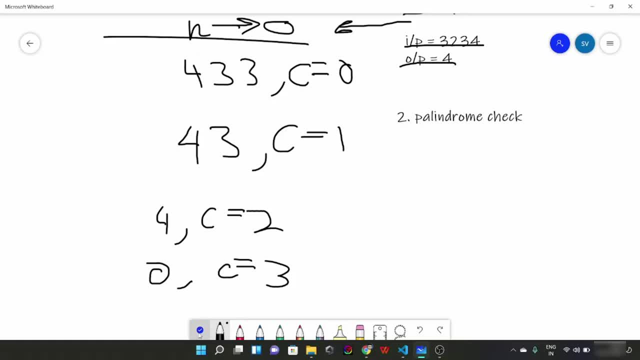 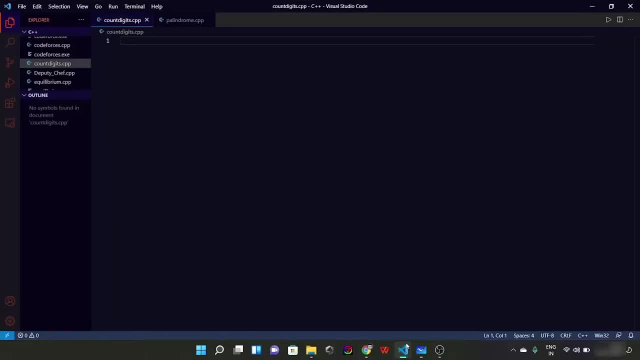 so this is the basic idea of this solution: to find the number of digits in any given number. all right, now let's try to code this solution. okay, so first of all let's upload our header file. then main space is 3d. let's make a main function. 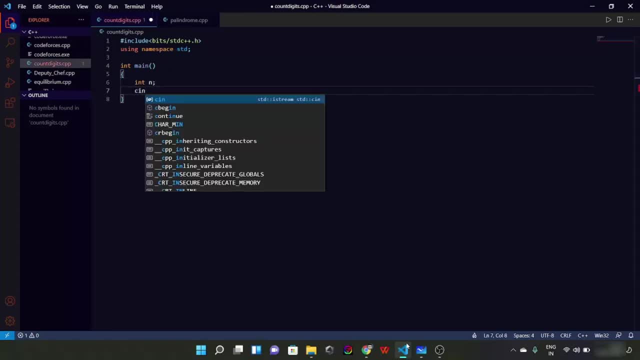 so we will have n and we have a user defined it, all right. and then we are going to see how count digit. all right, now let's make a function of by name count digits. by name count digit. all right, let's open up our image. let's park n as its parameter. 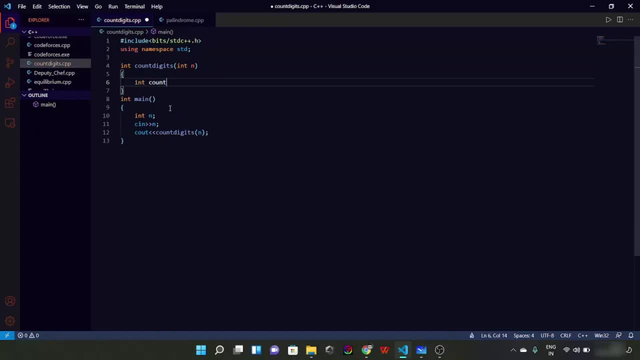 okay, now let's have our count variable initially zero. right now we'll make a loop that state that there are, and as long as t is more than zero, this loop is zero, and so that is our all, our number, and then we will just save it for the next step. 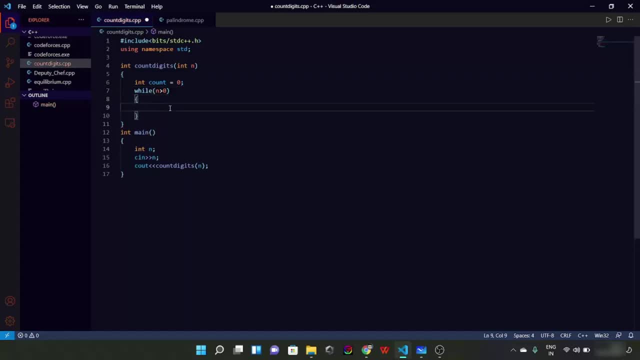 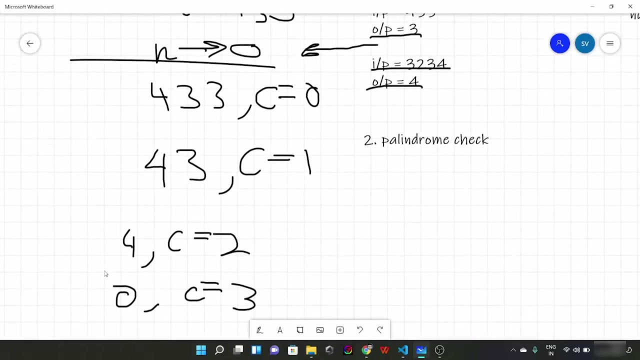 its loop is going to return. Now, what we are going to do is what did I tell you? we will divide n continuously and every time we are going to increment, count and count will be the number of digits and we will return. count right, c here, c is our count. yeah, c after. 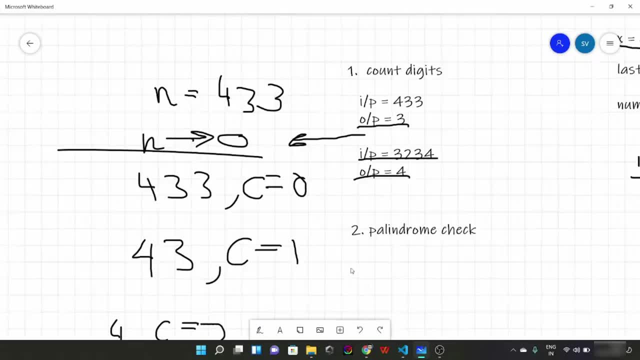 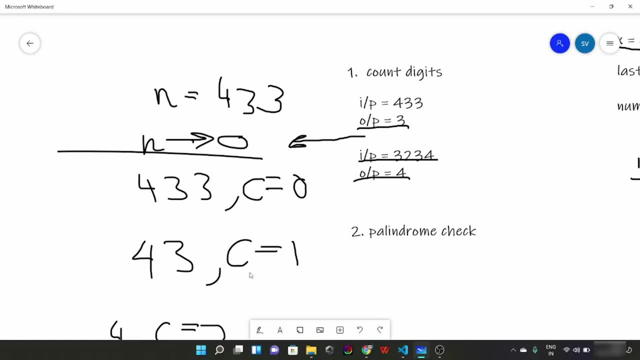 when the loop ends, c is 3 and if we see the output, output is also 3 and it is the correct solution. So c is going to be the number of digits, right? So this is going to be our function. let's leave it. 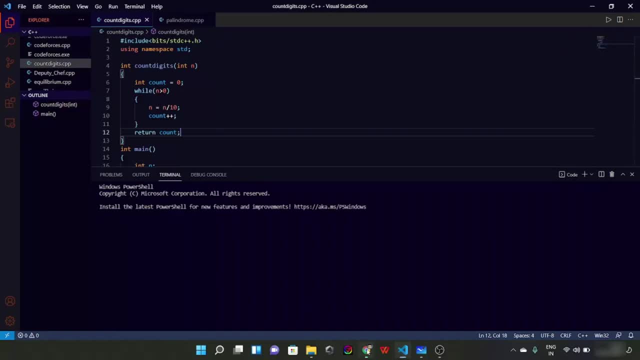 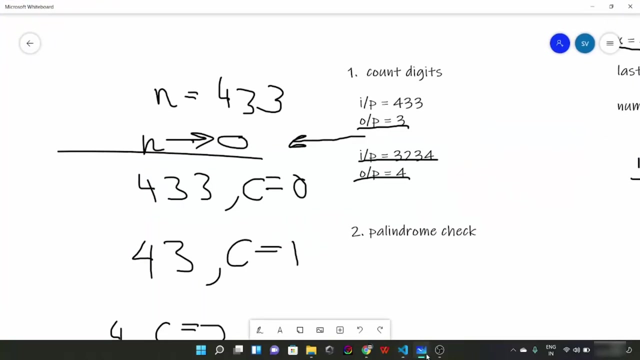 Let's try to run it. Let's change it for example 433, and we will write 433, c. we are going to return and c right, clear Now. next time, let's you know p323, code here: p323.. 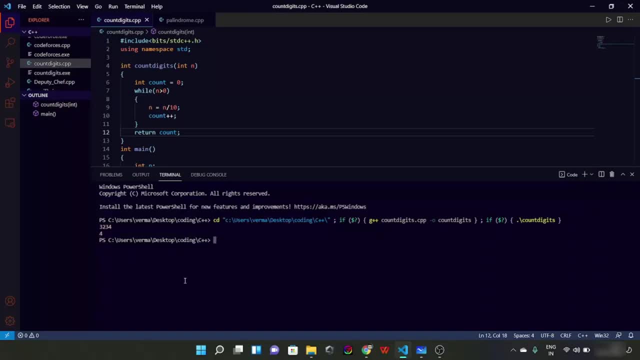 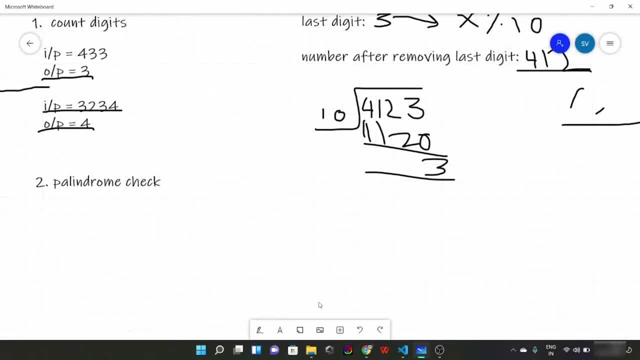 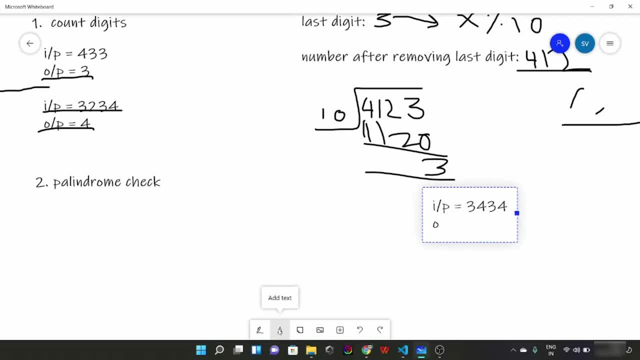 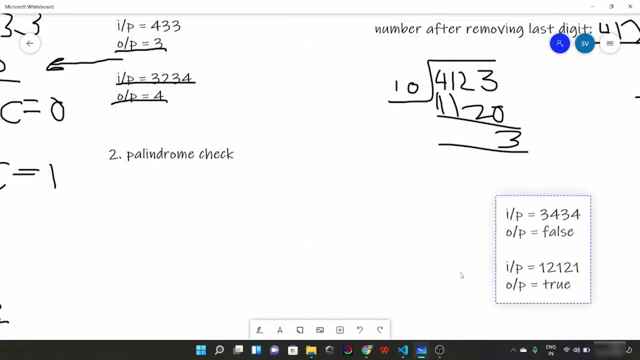 then our output is gonna be false, and if input is 1 to 1 to 1, output is gonna be true. alright, Now you might be wondering: what is palindrome here? So let's understand what is a palindrome. So palindrome means if I read a number from left to right and if I read a number from 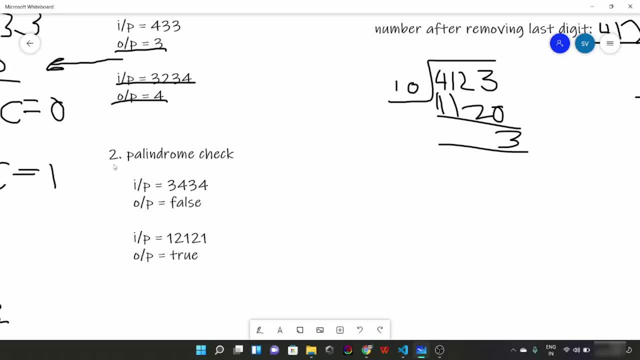 right to left, then answer will be same. alright. For example, let's see here: if we read it from left to right, it's gonna be 3434, right, And if I'm going to read it from right to left, it's gonna be 4343.. 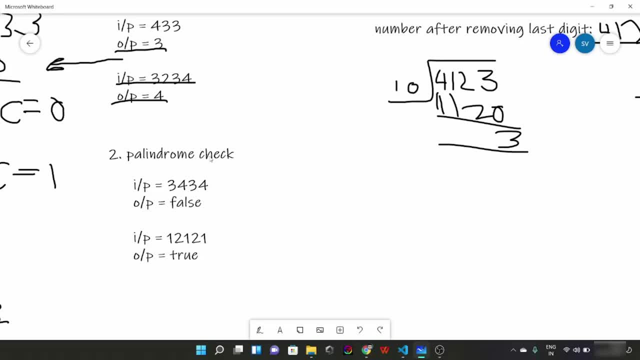 So 3434 and 4343 are not equal, since the output would be false. alright, And suppose, at any point now let's go to another example. so, for example, 12121, alright, If I read it from left to right, it's gonna be 12121, alright. 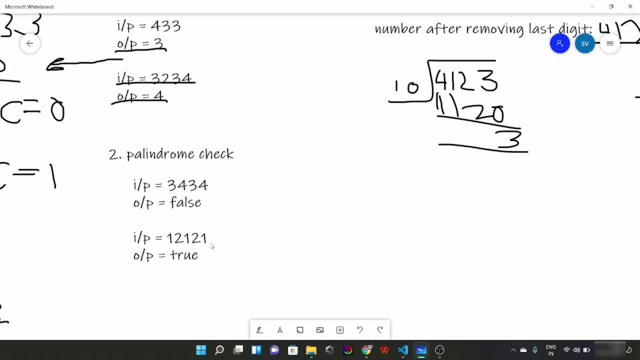 And if I'm going to read it from right to left, it's gonna be 12121. Hence 12121 and 12121 are equal. Hence output is going to be true right Now again. pause for 2 minutes and think for the solution here. alright. 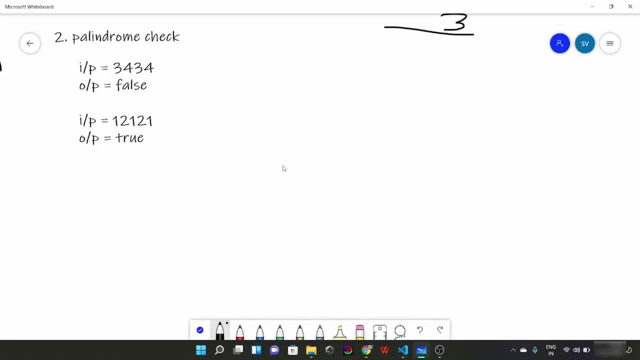 So let's jump to solution. What you have to do is what you can do here is you can have a variable, a rev. alright, there is a variable. You will store the reverse of the number. alright, In this case, you will store the reverse of the number as 4343, right? 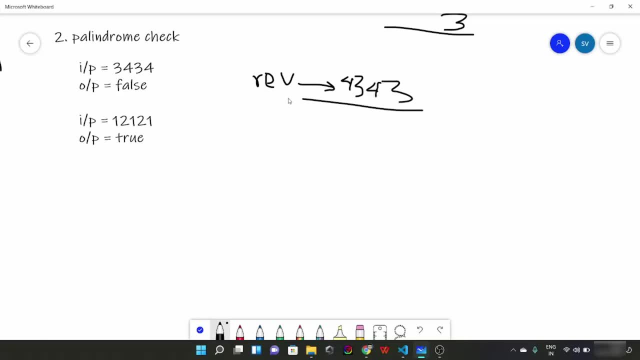 Here, here, reverse will be what? 12121, right? And then you compare reverse. Reverse with the original number, alright with the original number, And if reverse is equal to original number, we will return true, like in this case, original. 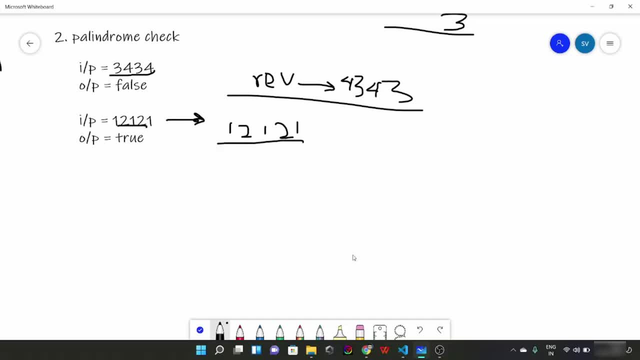 number is this and reverse number is this. both are same. So we will, you know, return true And here yes. here the reverse number is not equal to the original number. hence we will return false, alright. Now the main question arises is how you will find the reverse of a number. alright. 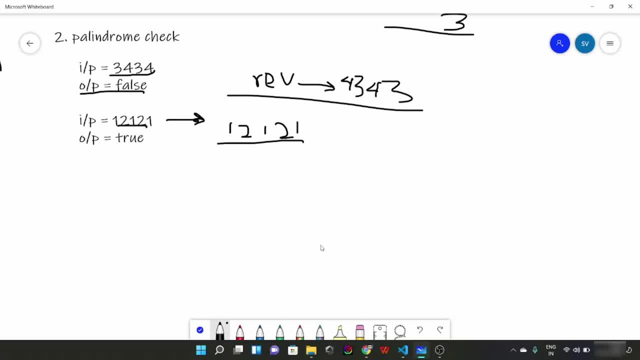 So here, the percent sign, which we studied earlier in this video, will come in handy. alright, What we will do here is that we will use a loop here, So we will use a loop here, So we will use a loop here. 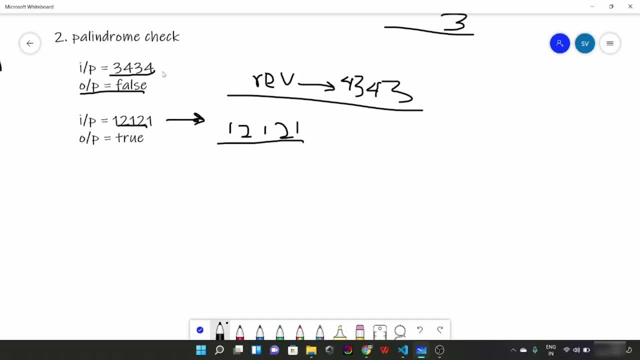 So we will use a loop here And what we will do is we will find the units digit, the last digit. alright, Okay, let's have a dry run, so you will understand it. What I am trying to say is the number is what? 3434, right. 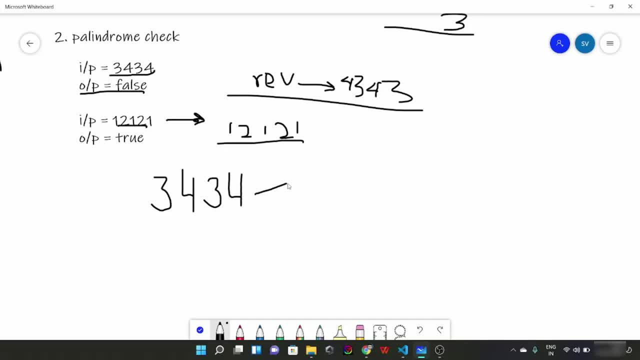 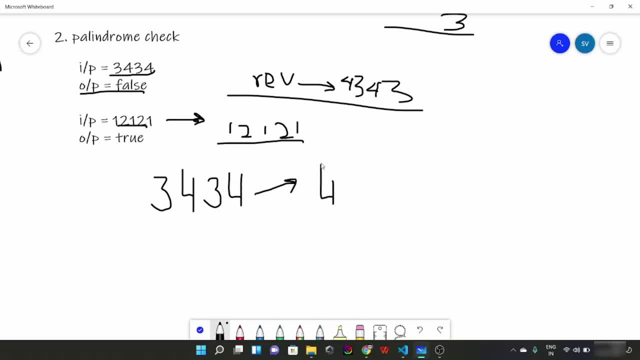 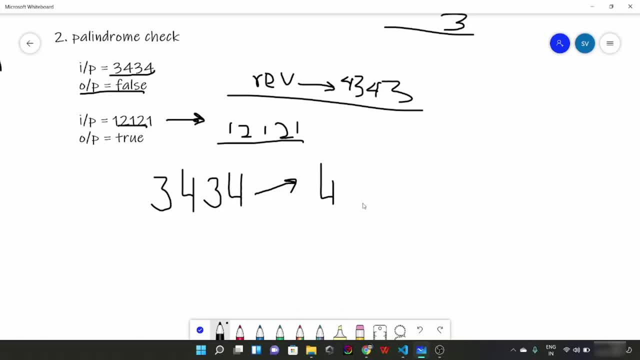 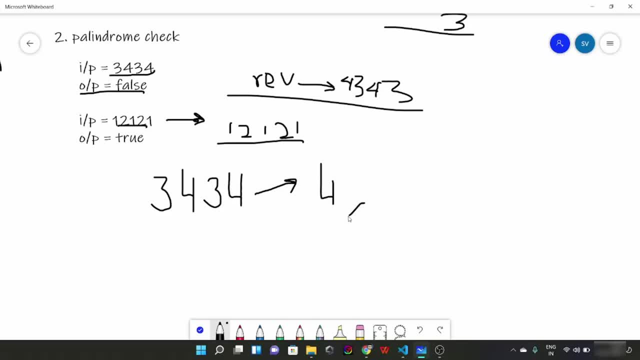 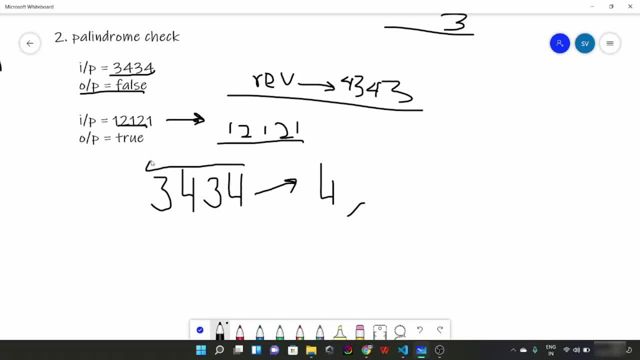 So if you have to read it from here to here, you need to find all the digits from right to left, one by one. So first digit comes out to be 4.. Now, if I have to find next right to left digit, what I have to do 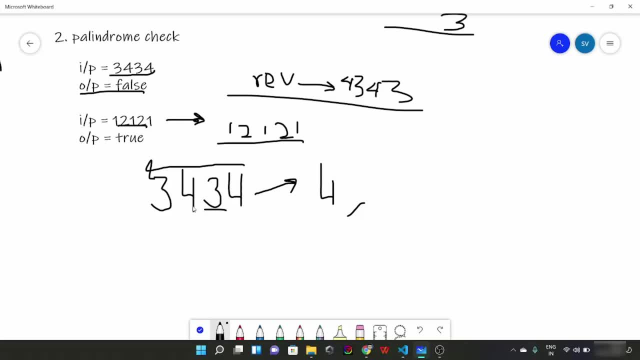 I have to eliminate this one. So what you will do, You will divide this number by 10, hence this number would come yes, Now here. what you will do is you will find this digit, units, digit here, which is going: 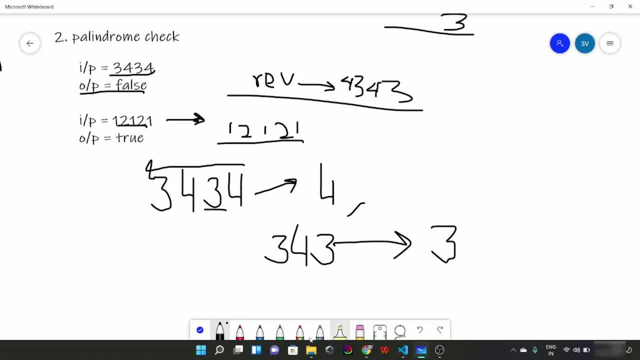 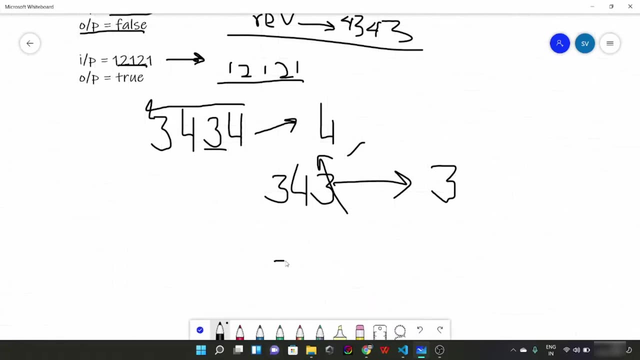 to be 3.. And now what you will do is to find this digit. you will eliminate this one, Right? You will eliminate this one, so your new number becomes 34,. right Now, here, your new digit is going to be what? 3,, sorry, 4,. this one. 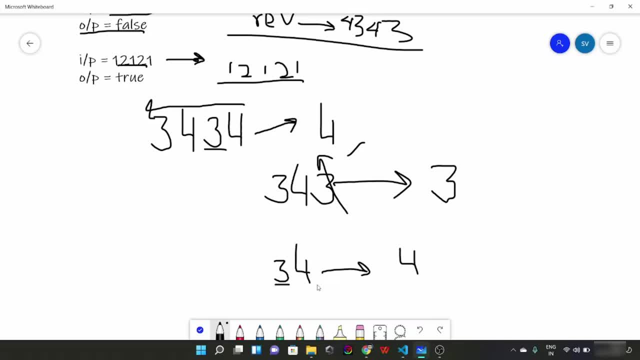 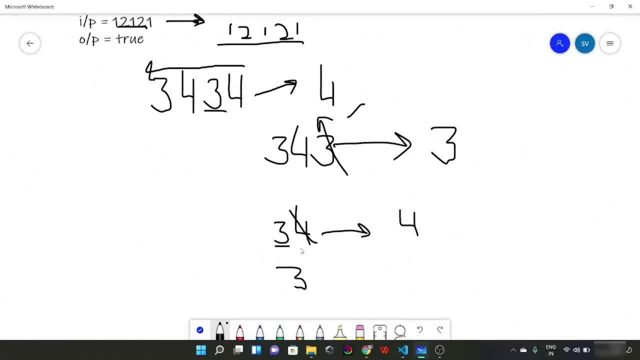 Now, if I have to find the next right to left digit, I have to eliminate this one. yes, I have to eliminate this one right Now. it will come after the 3. To find this digit. what I will do again is, you know, I will have this digit and now I. 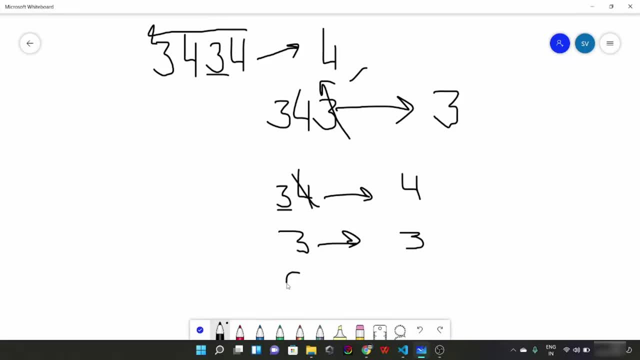 will again, you know, divide it by 10, so it comes out to be 0.. As soon as we reach 0, it will come out of the loop. Okay, As soon as we reach 0, it will come out of the loop. 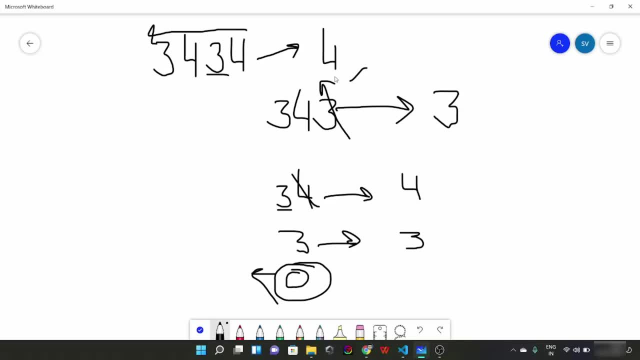 Okay, So 4, 3, 4, 3.. This is going to be, you know, this way we are going to have a reverse number And what we have to do is, if I directly add, you know these numbers, so these will. 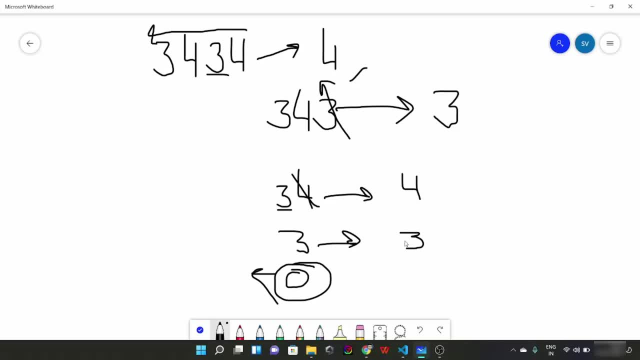 result in what 4 plus 3 is 7,, 7 plus 4, 11,, 14.. Right, that every time when i add this number to this reverse variable, i multiply the reverse variable by 10.. all right. so here it would be. you know, 4 into 10, 40, right? and then when i add 3 here 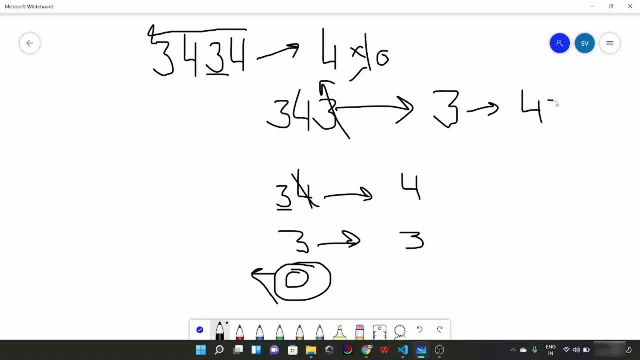 it is going to be worth 43.. now here i'll again multiply it with 10. it is going to be worth 430. then i'll add this number, it will become 434. and again i'll multiply this with 10 and then add this and it becomes 4: 3, 4, 3. 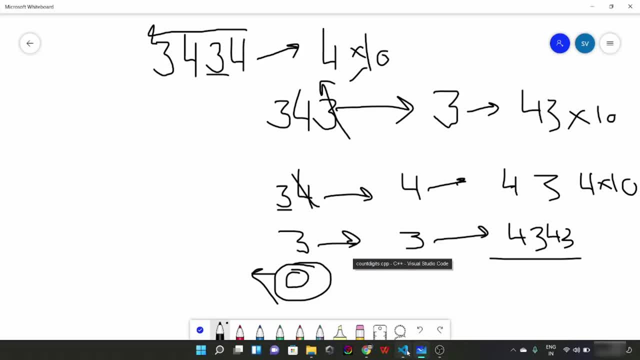 right. so this is going to be the main idea of how to do this question. first, um, for the basic um idea is to find the reverse of this number and how to find the reverse of this number. i told you about it all right now. let's, let's try to code this program. 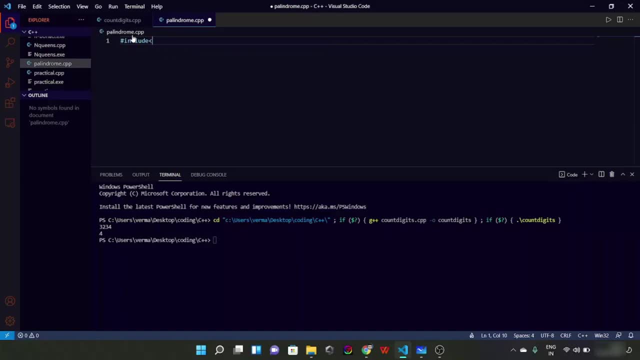 so we'll add a header file here first of all and then name space std. right, we have our main variable, main function. we have variable l. we'll take it from user um. so let's name our functional style all right. style n: cout true, else cout false. all right, 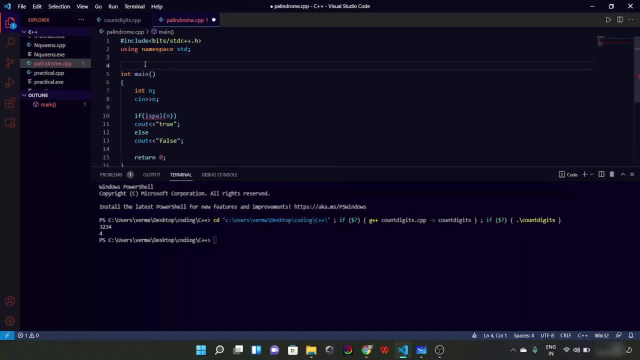 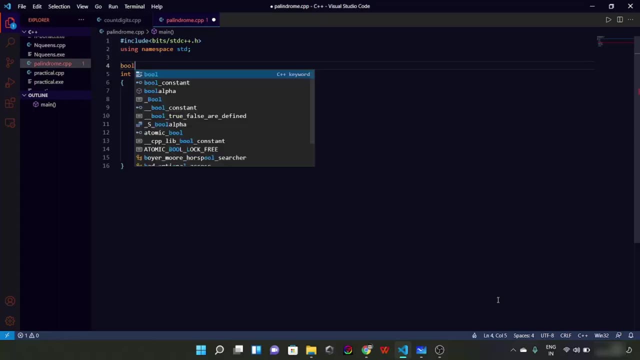 now let's have a s file function. we'll have it as a boolean function. all right, i am hoping you might be knowing what is a boolean function. so what boolean function does is either returns true or false. so by this condition of s file n, this means that if this 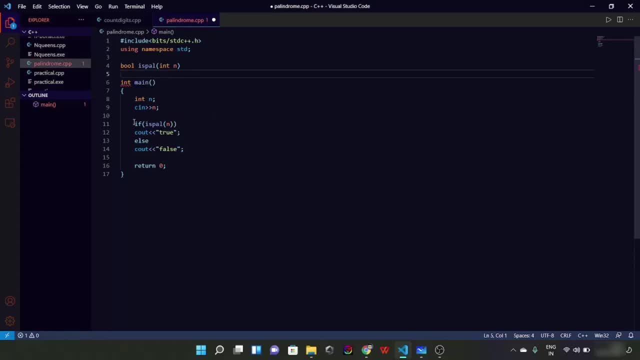 function returns true, then we will see our true and else we will see our false. okay, So now let's have our reverse, which I will go to 0, where you know we will store the reverse number. We have a temporary variable on which we operate of doing, you know that, divide operation. 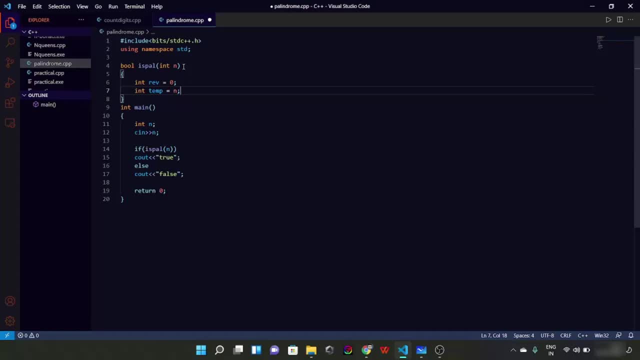 because see, if you do it on n, then how we will compare it with reverse number, because then n will become 0 after the while do. Hence, we will have a temporary variable which will have a same value as 0. Okay, And we will do the operations on it. I will try it. we declare it temporary, which is equal. 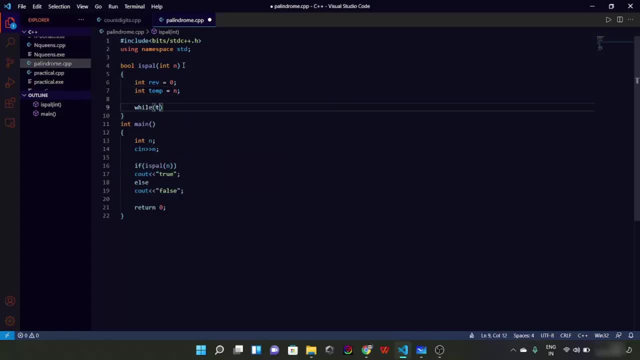 to 1 and what we are going to do is find 10 more than 0, let's have, let's have it unit digit. So unit digit as 10 percent 10, right, Or we did. I tell you what we will store in rev: we will have rev percent 10 plus unit. 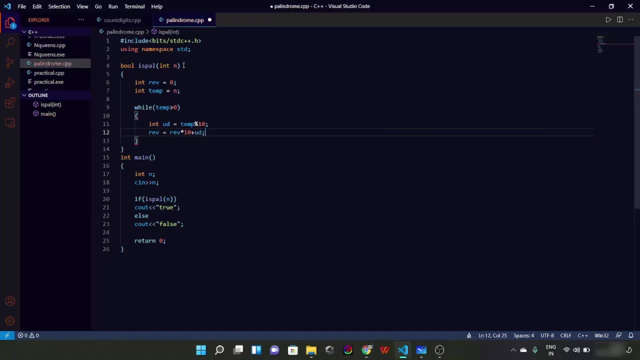 digit. All right, Okay. So now let's see what we are going to do. we are going to have unit digit as 10 plus unit digit, Okay, And then we will have 10 plus 10 by 10.. All right. 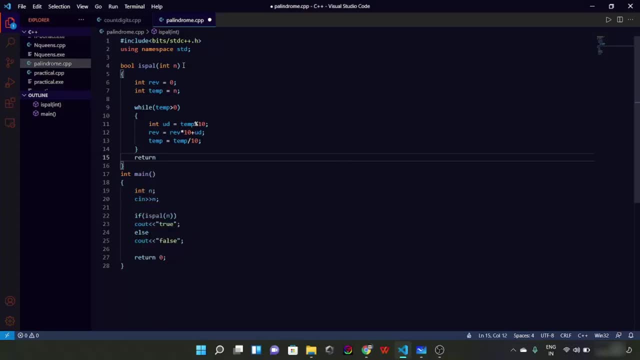 And then what we will return here we will return: n is equal to is equal to. reverse is equal to is equal to n. So what this line is going to return is that we will check the return. If this is true, then we will, you know, return true and else we will return false.